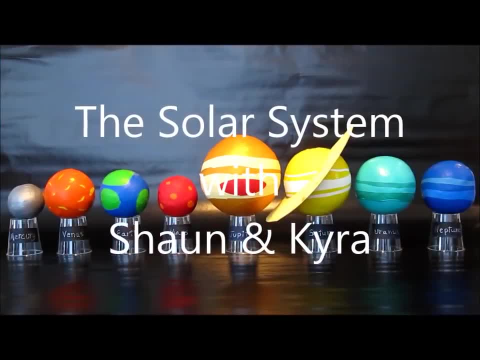 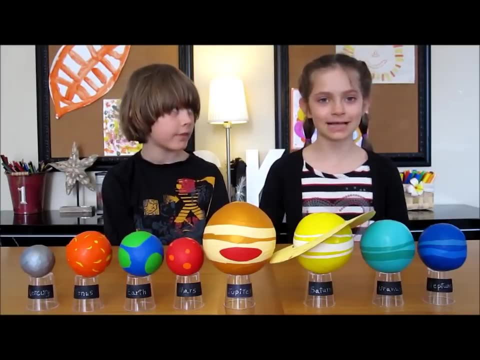 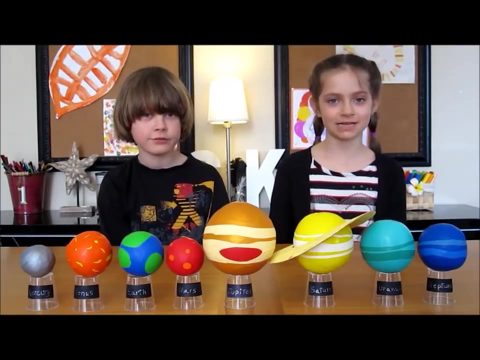 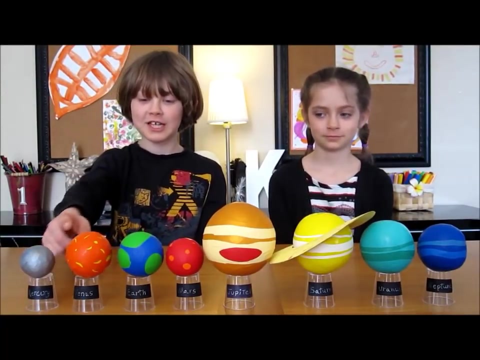 Hello everyone. In the last video we did the rice and balloon technique for the juggling balls and it gave us the idea to make the solar system. Our solar system is 8 planets: Mercury, Venus, Earth, Mars, Jupiter, Saturn, Uranus, Neptune. Mercury- Venus, Earth, Mars, Jupiter, Saturn, Uranus, Neptune. Mercury- Venus, Earth, Mars, Jupiter, Saturn, Uranus, Neptune. Let's start with the first planet, Mercury. Mercury is the smallest of the solar system. 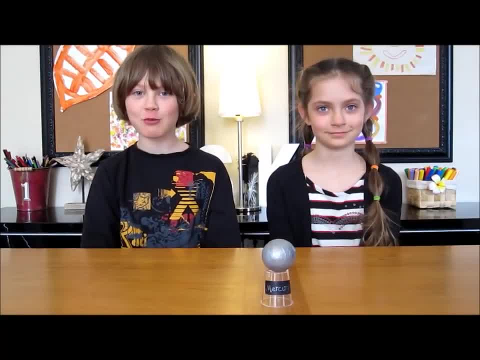 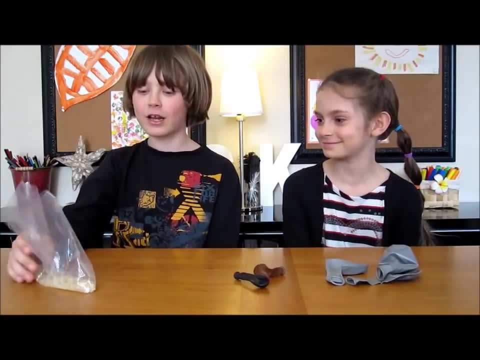 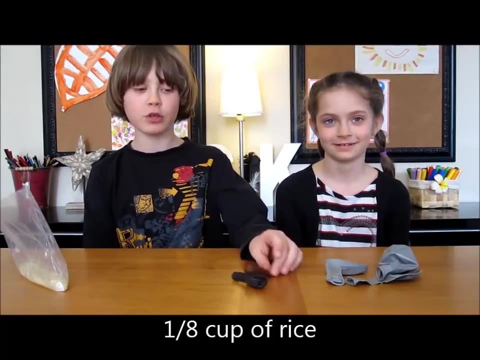 and it's the closest of the sun. It's a hot, rocky ball of iron with no moon. To do Mercury, take a small plastic bag and fill up with rice- one-eighth cup of rice- And then take two small balloons any color that you want, and for the gray take three. 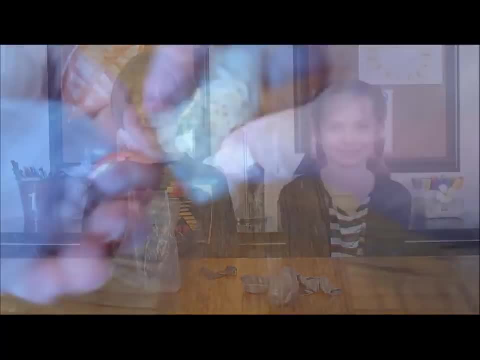 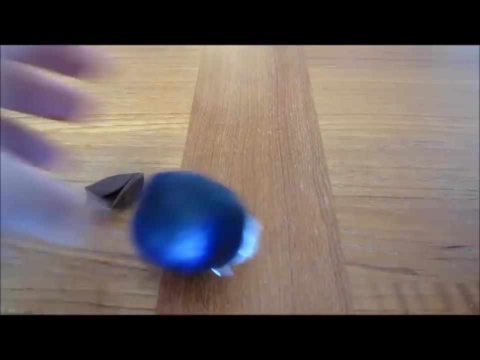 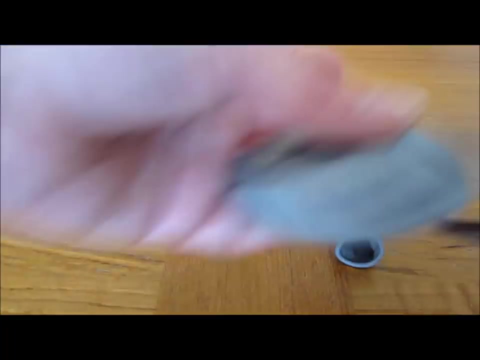 big balloons and cut the necks off To make Mercury. take a small plastic bag- one-eighth cup of rice, one-eighth cup of rice- and then take some balloons and fill up with rice- one-eighth cup of water. 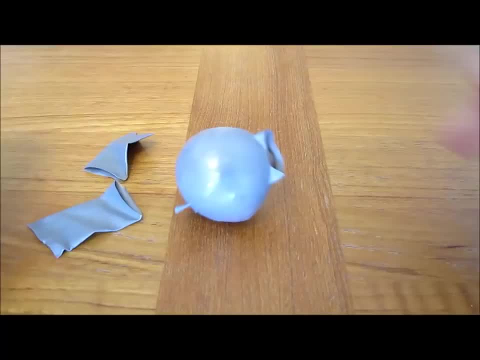 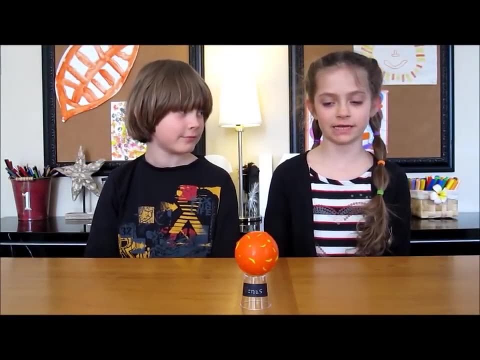 Take a small plastic bag, cover it with a clean towel and put a sheet of paper over it to make it easier to move. The second planet is Venus. It's the brightest and the hottest of the solar system. Venus is the same size as the Earth. its red color is the yellow and its yellow color is the 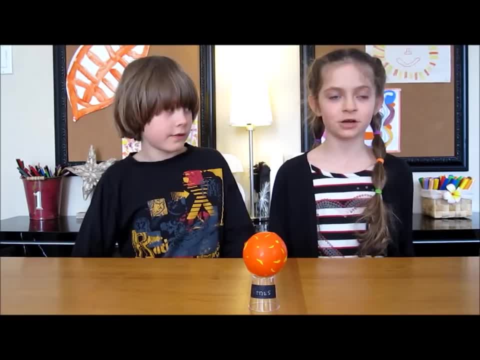 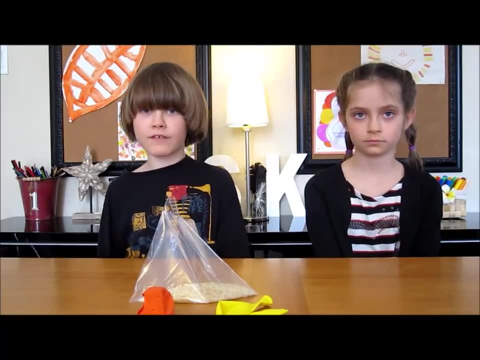 brown. Venus is the smallest of the solar systems. It has at least one planet and the, But it spins the other way and much more slowly than the Earth. For Venus, take a small bag and you need one third of a cup of rice. 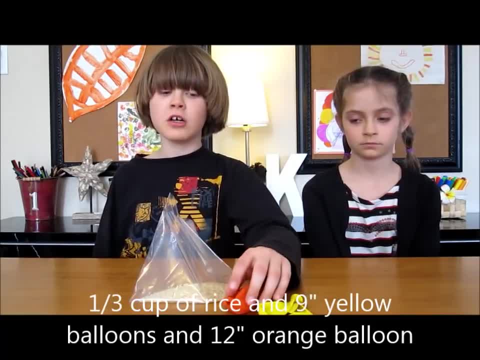 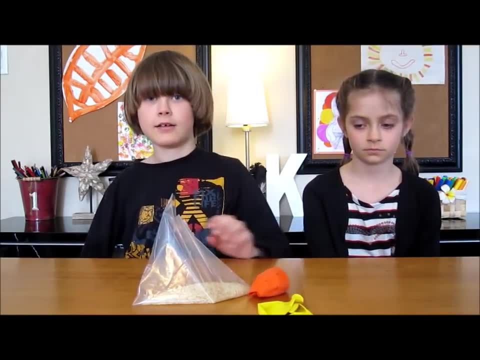 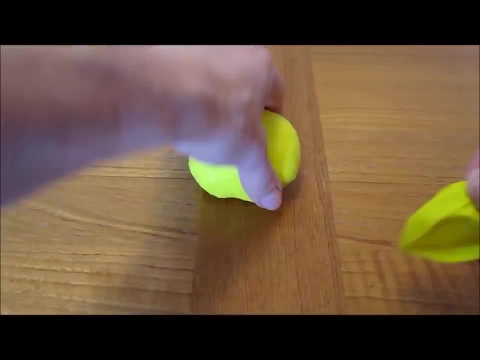 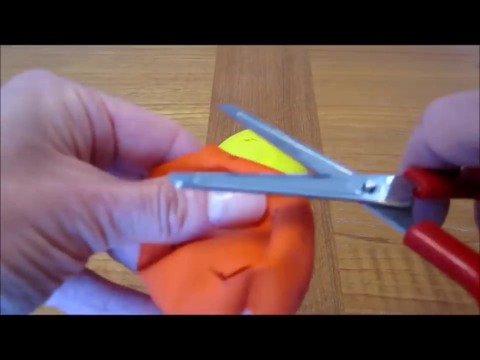 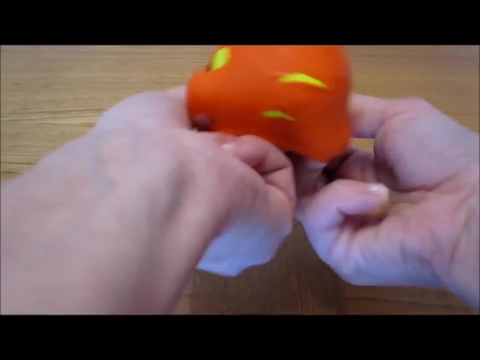 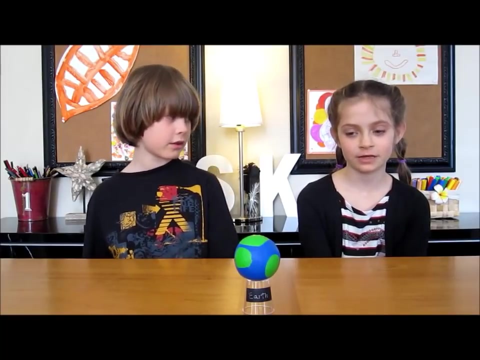 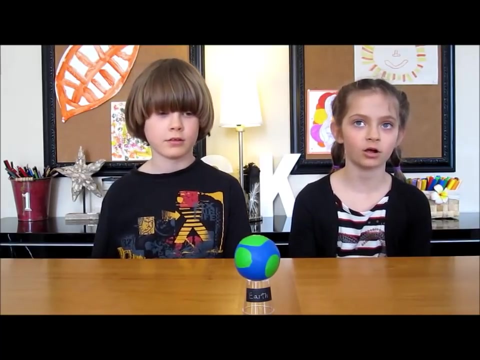 Take two yellow balloons and one orange. With the orange, cut the neck and make slits and holes inside to make the lava streams. The third planet is the Earth. The Earth has one moon and the Earth is covered with seas and lands and the land is called continents. 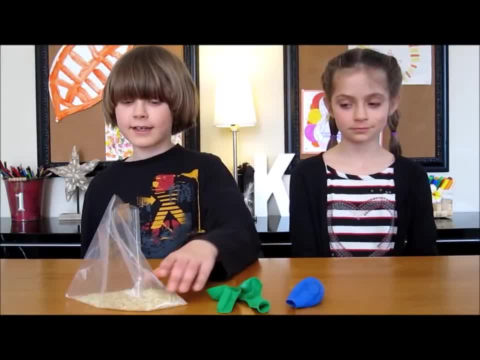 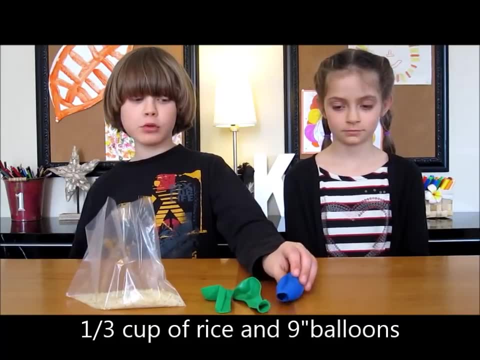 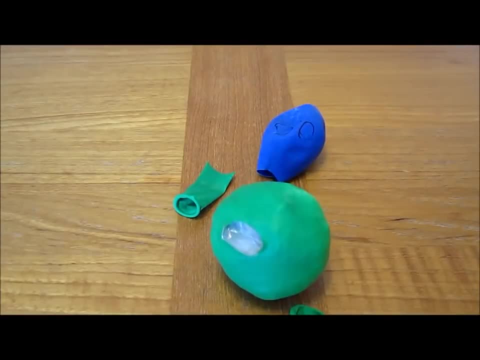 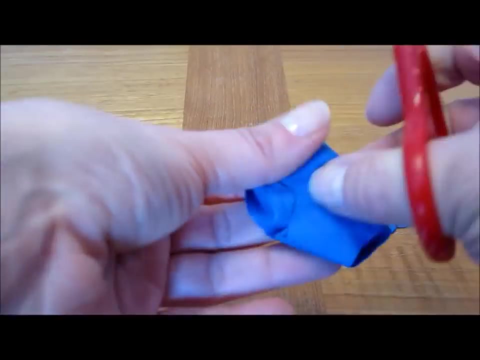 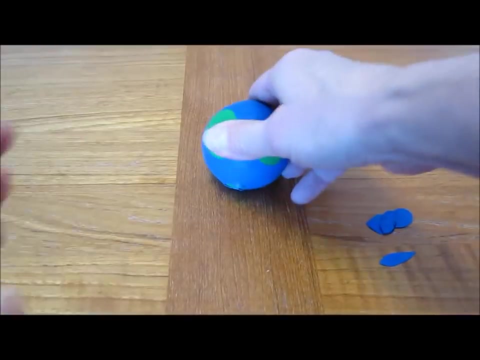 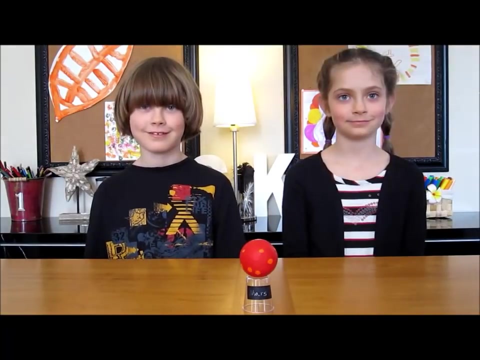 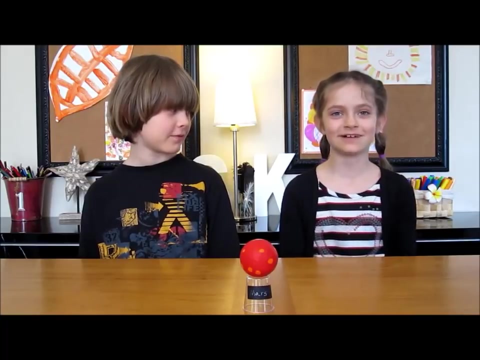 For the Earth. take a small bag of one third of rice, two green balloons, one blue balloon and cut four holes. The fourth planet is Mars, and it's a rocky red planet. Iron oxide is giving it its rust color. It has the highest mountains and the deepest valleys. 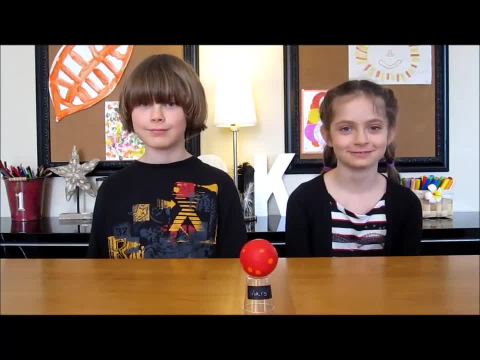 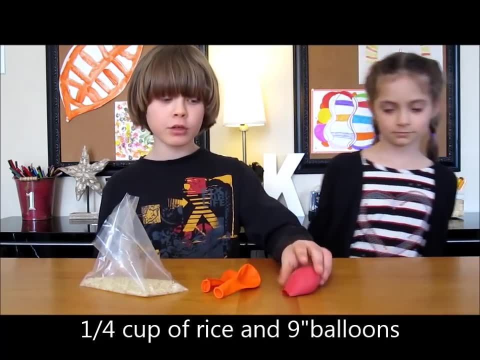 It's dry and cold and it has two moons To do planet Mars. use one quarter of rice, two orange balloons, one red balloon. cut the neck off and do the same thing on the other side. Take two little circles to do craters. 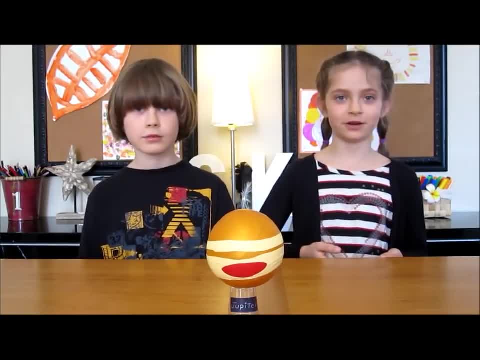 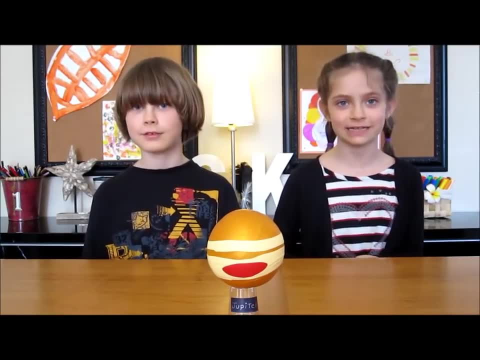 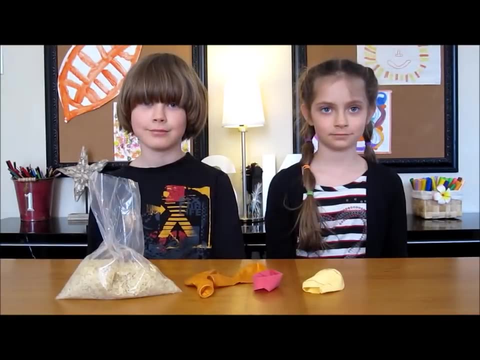 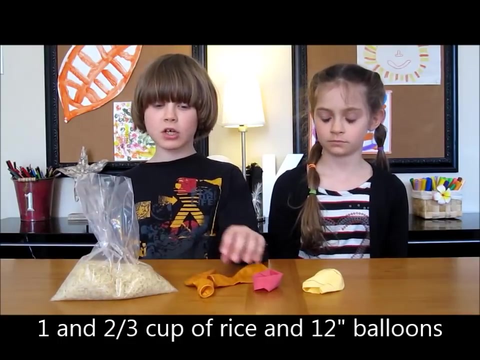 The fifth planet is Jupiter. Jupiter is a gas giant and it's the biggest planet of the solar system and the fastest. It has a great red spot larger than the Earth, created by a storm. To do Jupiter, take one cup and two thirds of rice, two gold balloons. 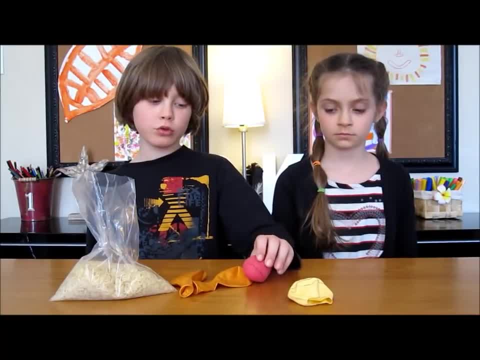 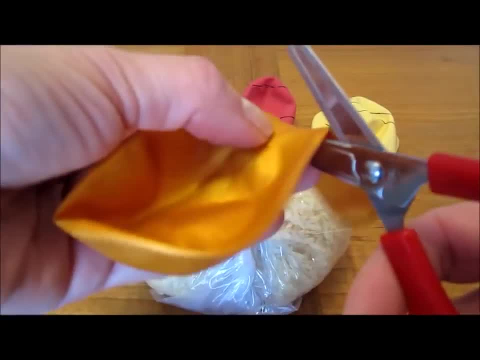 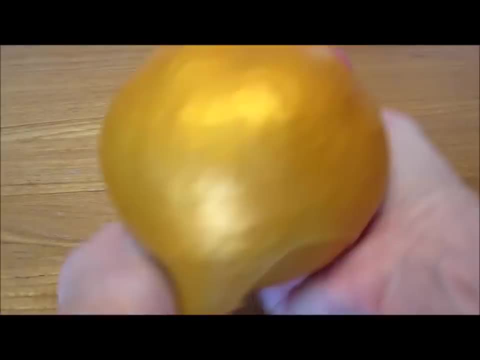 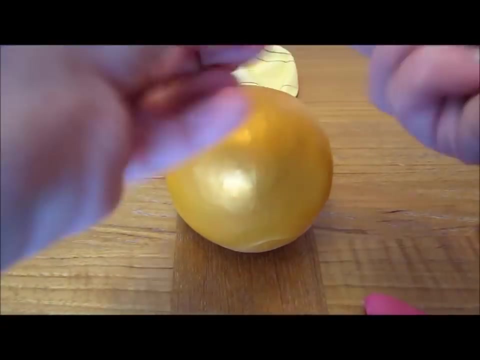 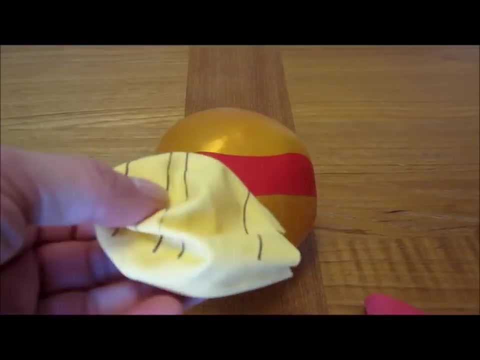 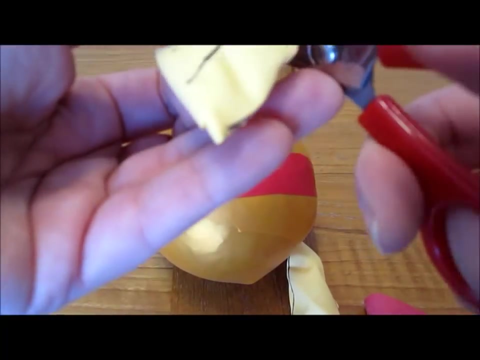 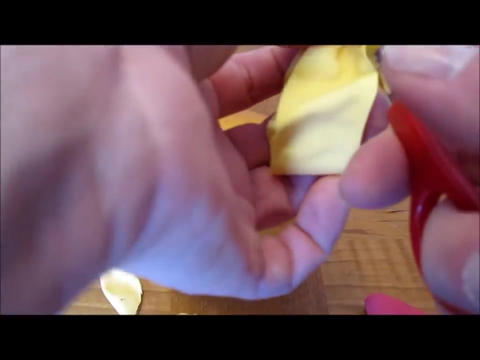 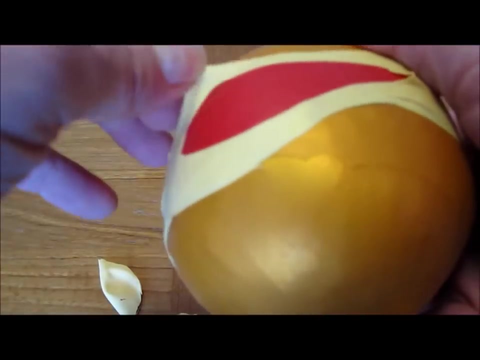 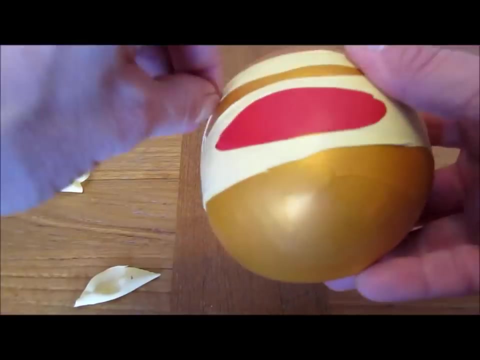 To do the great red spot. do a stripe in the red balloon and two stripes in the yellow balloon. Cut craters in the fourth planet. Place the craters With two stripes. I got a biglah balloon, Thank you. The sixth planet, Saturn, is another gas giant. 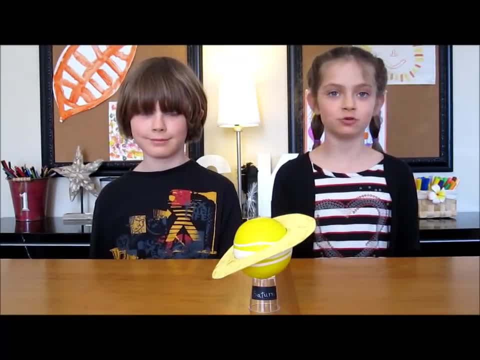 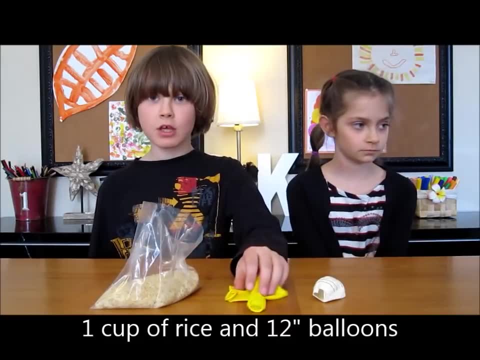 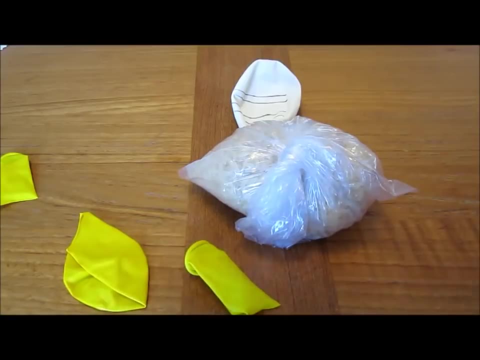 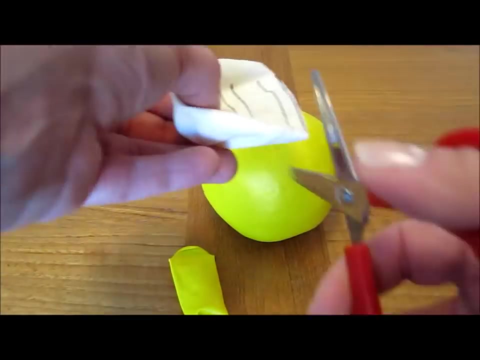 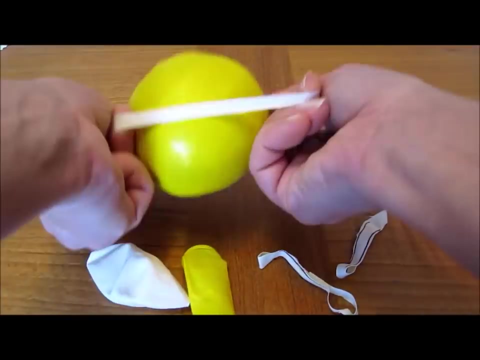 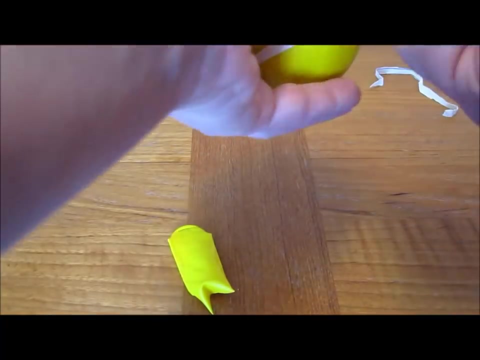 His rings are made of rocks and ice and his biggest moon is called Titan. To do the planet Saturn, do one cup of rice, two yellow balloons and do stripes in a white balloon. To do the ring, use a plastic lid. 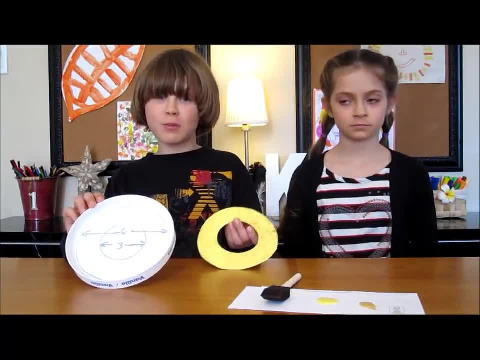 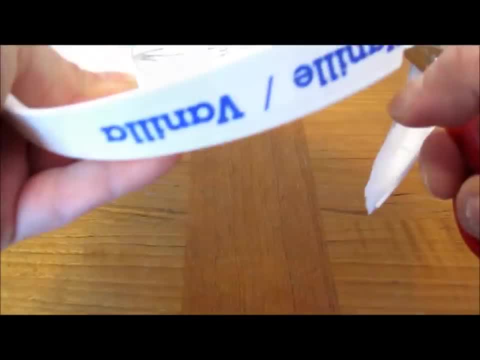 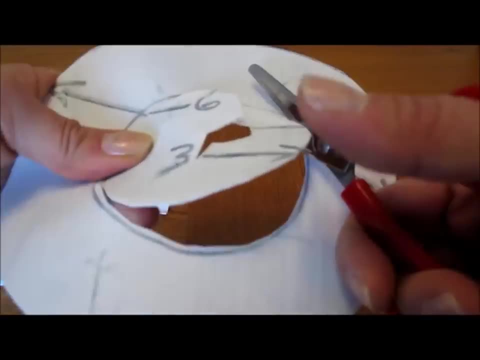 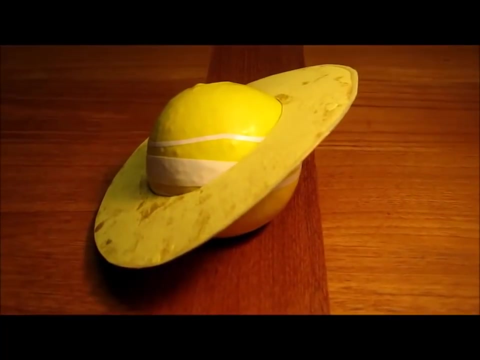 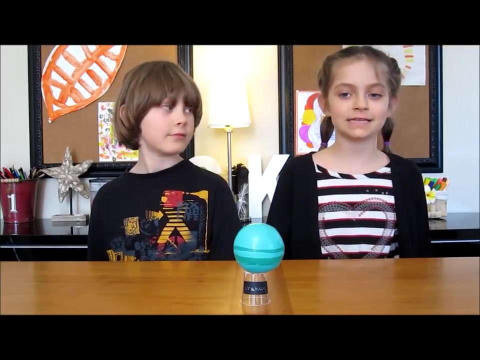 Do a six-inch circle and a three-inch smaller circle in the middle and paint it in gold and yellow. The seventh planet is Uranus. It's an icy gas giant, It's the coldest planet of the solar system and it has a turquoise color. 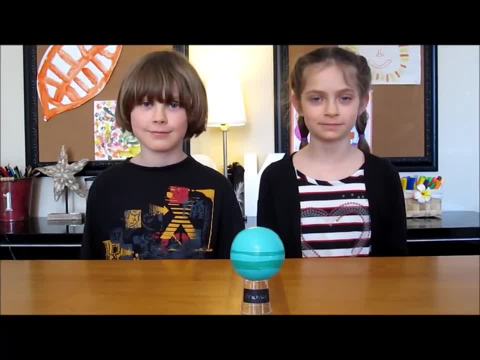 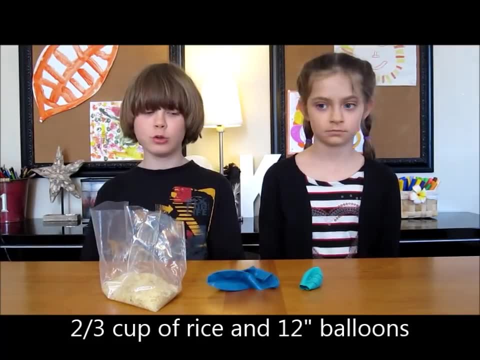 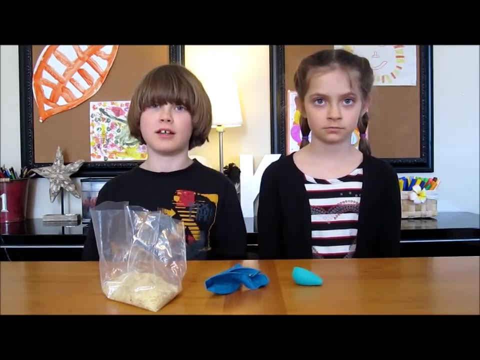 It's the coldest planet of the solar system and it has a turquoise color. It has 27 moons. To do Uranus, use two-thirds of a cup of rice, Use two-tailed balloons and a turquoise balloon and cut stripes on it. 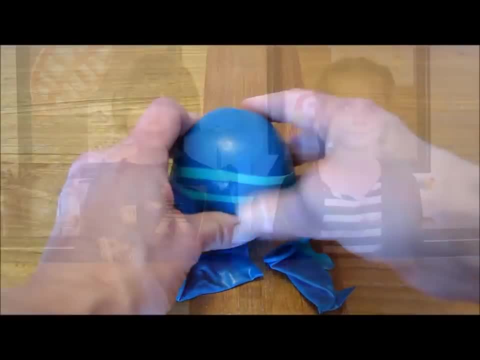 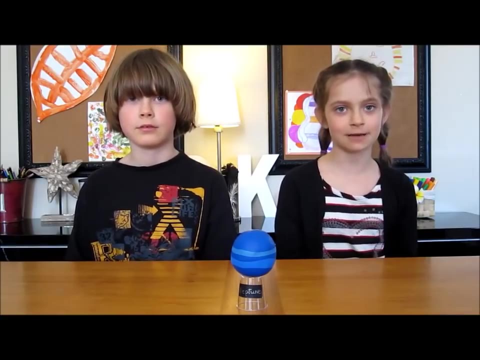 Use two-thirds of a cup of rice, two dark balloons, one lighter blue balloon and do stripes. And finally, the last planet and the eighth planet is Neptune. It's also a gas giant and it's windy and it's very cold. 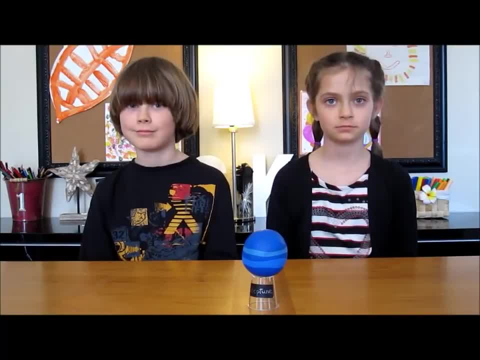 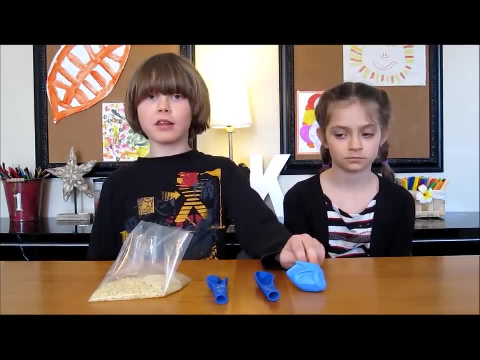 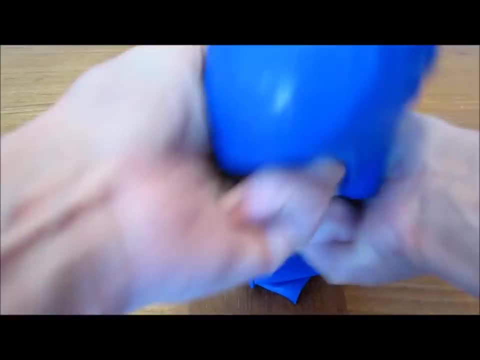 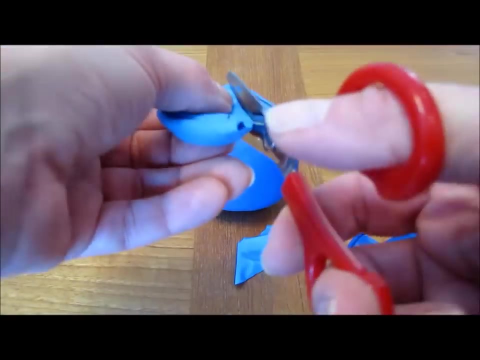 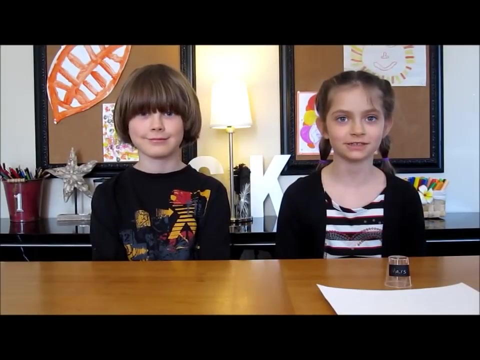 And it has also very big storms. To do Neptune, use one-half cup of rice, two dark balloons, one lighter blue balloon and do stripes. For our little stand we used smaller plastic cups and we wrote the names of the planets on it. Thanks for watching and we'll see you next time. Bye, Bye.